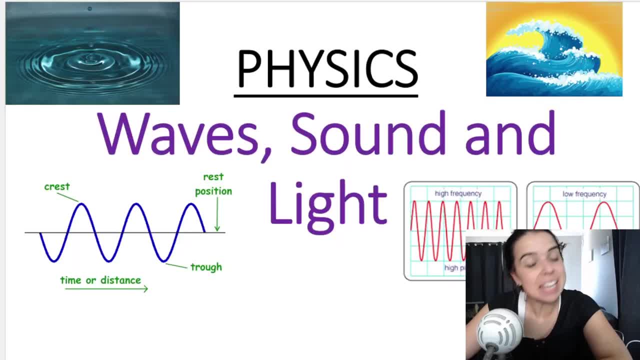 practice calculations themselves. Let's go. This topic in physics has to do with waves, sound and light. We will discuss sound in the context of sound being a wave, and light in the context of light exhibiting both wave and a particle nature. Now remember the main focus of this chapter. 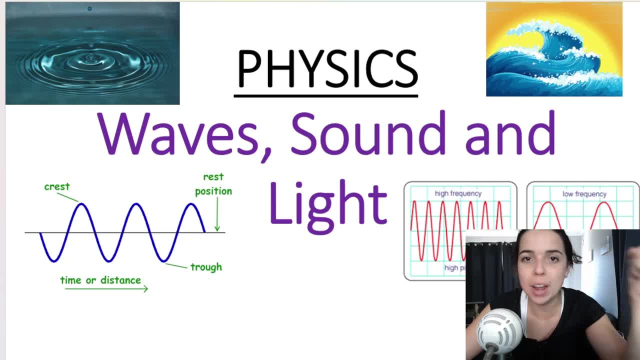 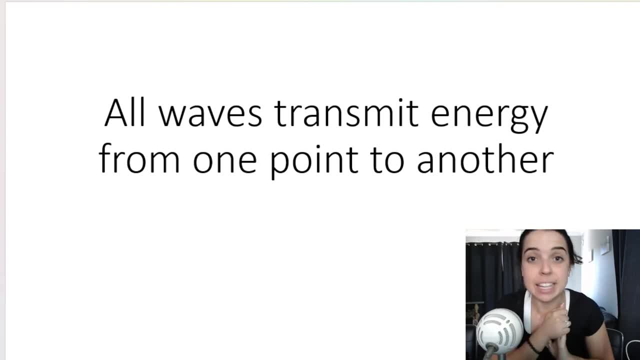 is waves. What is the most important thing to know about waves? All waves, whether they are transverse waves, longitudinal waves, electromagnetic radiation- all waves transmit, so essentially carry Energy from one point to another. Now this video is basically just going to focus on what are the 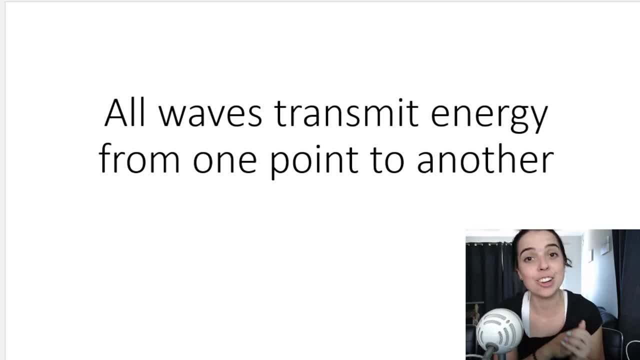 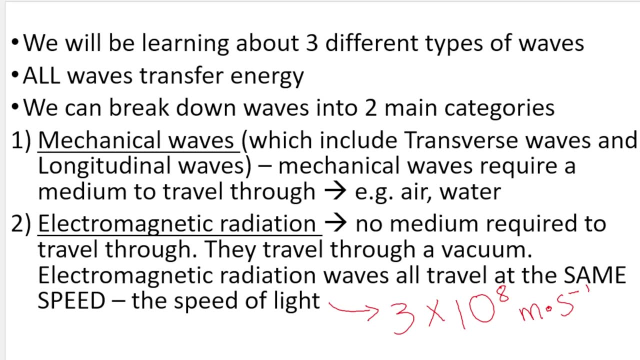 three different types of ways that we will be learning about in grade 10.. You can see a little bit of a summary on the screen behind me. Like I said, we'll be learning about three different types of waves. All waves transfer energy and we can essentially break down waves into two main. 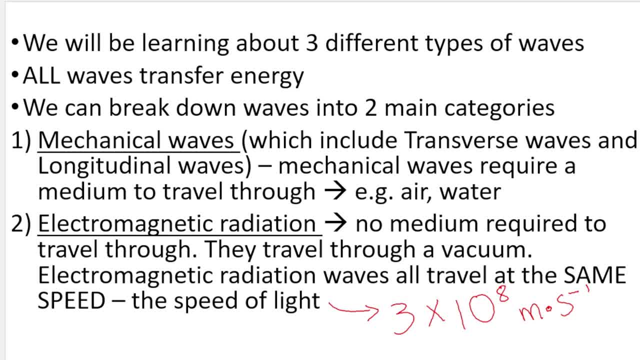 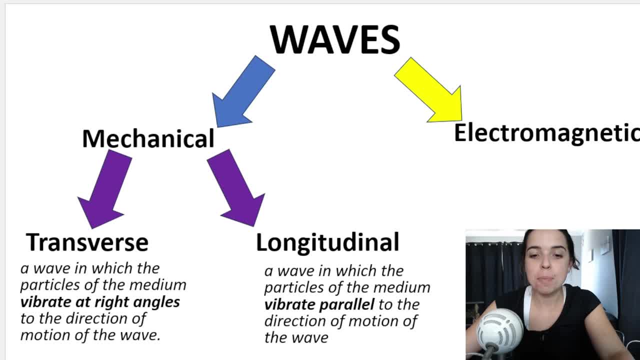 categories. We've got mechanical waves and electromagnetic radiation. I like to think of it like a wave transfer. I like to think of it like a wave transfer. I like to think of it like a flow chart, like this. So we've got waves. Remember, all waves transmit energy can be broken down into. 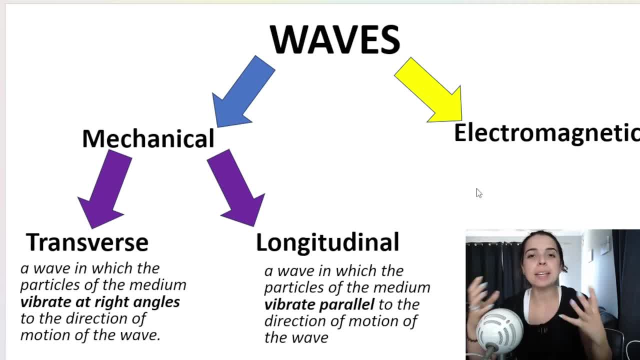 mechanical waves and electromagnetic waves, and under mechanical waves we have transfers and longitudinal waves. So those are the three that I was talking about: Transfers, longitudinal and electromagnetic. Now, what does mechanical mean? Let's just take a step back and focus on that. 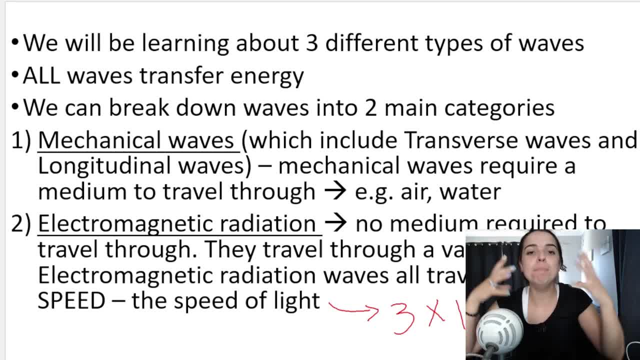 Mechanical waves are waves which require a medium to travel through, So the reason why you can hear my voice is because my voice is travelling through sound waves and it's travelling through the air. So the air is an example of a medium through which longitudinal waves travel, and 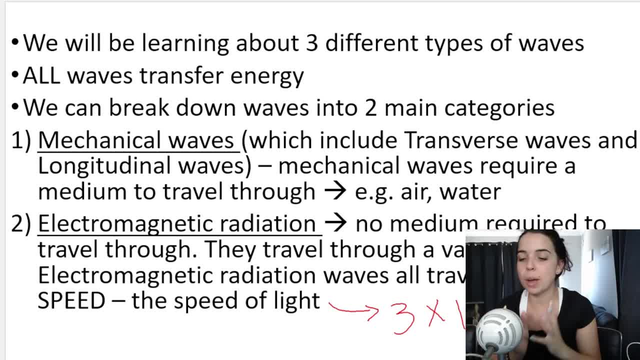 transverse waves. Water, that's another medium. So mechanical waves. how we can distinguish them or identify them is they are waves that require a medium to travel through, and those would be transverse waves and longitudinal waves. Electromagnetic radiation, which is the third. 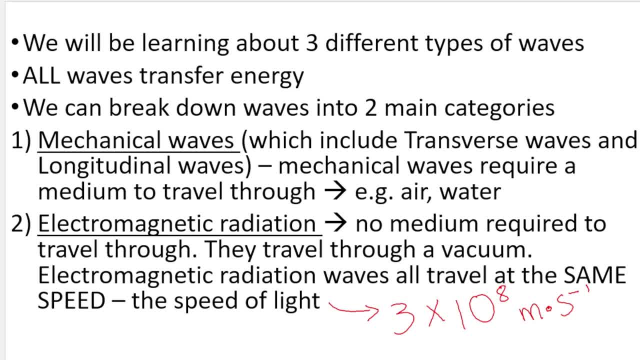 its own. They do not require a medium to travel through. They travel through a vacuum, which means they can travel through space. they can travel through incredibly long distances and they all travel at the same speed. That's what makes electromagnetic radiation special. They don't. 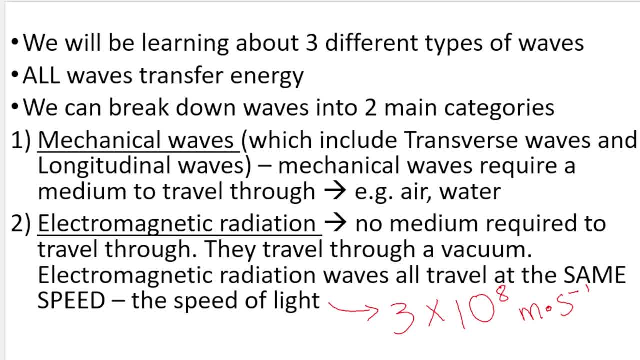 need a medium to travel through. they can all travel through a vacuum and they all travel at the same speed and that is the speed of light. and I've put the speed of light over there: 3 times 10 to the 8 meters per second. That is a gigantic number, Remember: 3 times 10 to the 8, times 10 to 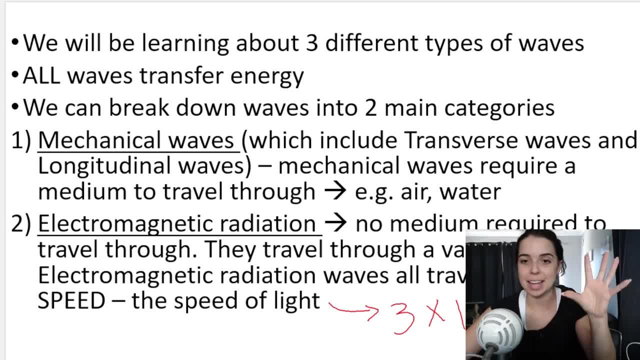 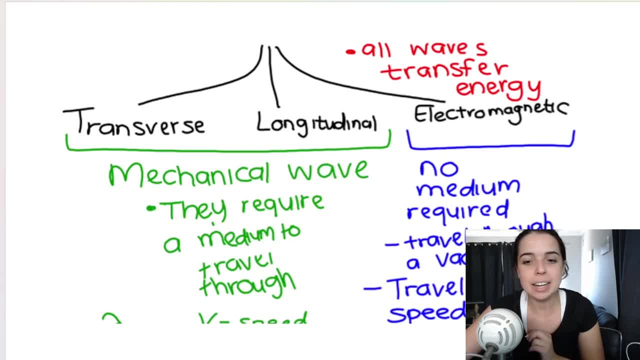 the 8,. that's scientific notation. That is insane. Think about that number, it is crazy. So that's the difference between mechanical and electromagnetic radiation. Again, here's another summary. let me move myself out the way so you can see Mechanical waves, those two electromagnetic. 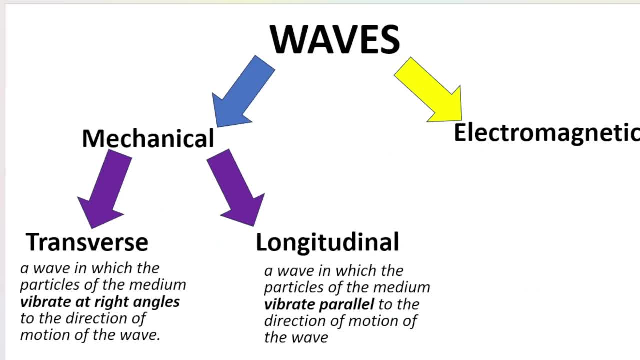 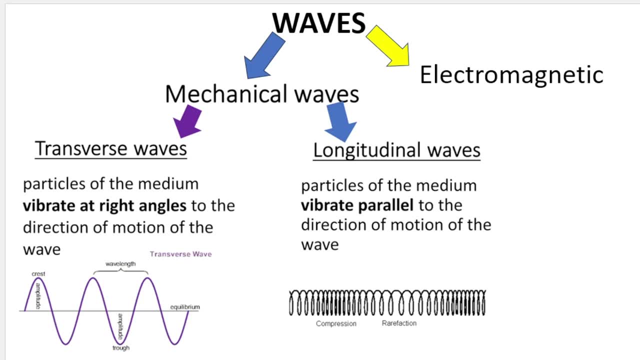 waves. So as long as you have one of those summaries down in your book, you should be fine. And here's a final way that I will summarize the differences between these waves. Now, electromagnetic radiation: remember, they're special, They do not require a medium to travel. 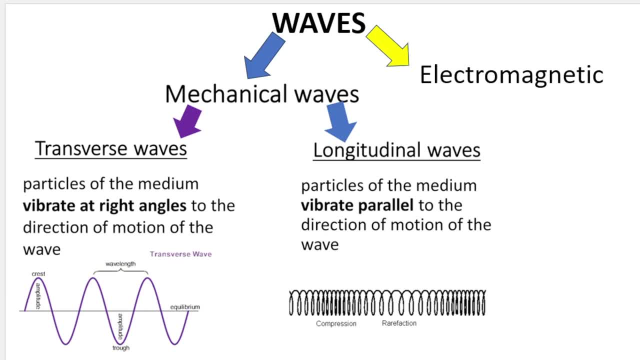 through. We will discuss those at a later stage. And then we have mechanical waves and the difference between those waves. it has to do with the vibrations or the movements of their particles. Now take a look at transverse waves. Here's an example of a transverse wave. Here's a 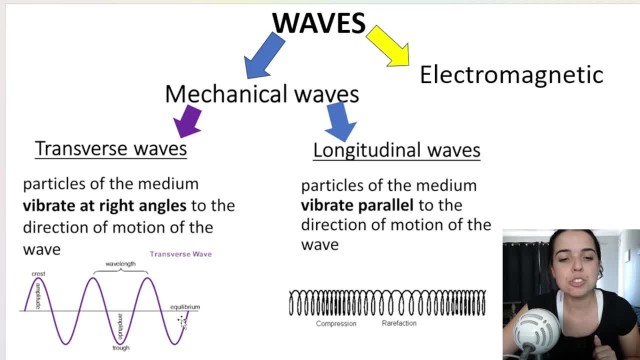 different example of a transverse wave. Here's a different example of a transverse wave. Here's a diagram representing a transverse wave. And what makes a transverse wave unique is that the particles of the medium- so remember, the medium is like the air or the water- vibrate or move at. 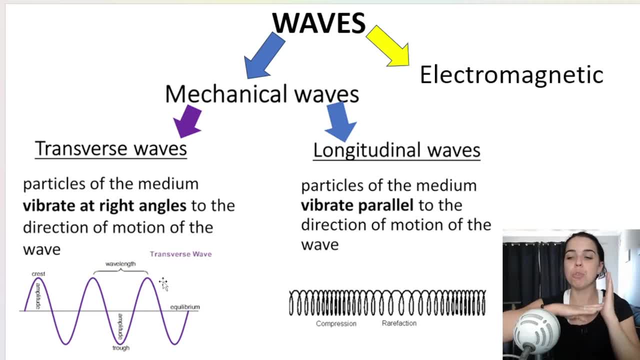 right angles to the direction of the motion of the wave. So what that means is that, for example, if this wave is moving to the right- sorry, that is very skew- then the particles will move at right angles, so they will move up and down, So the particles vibrate. 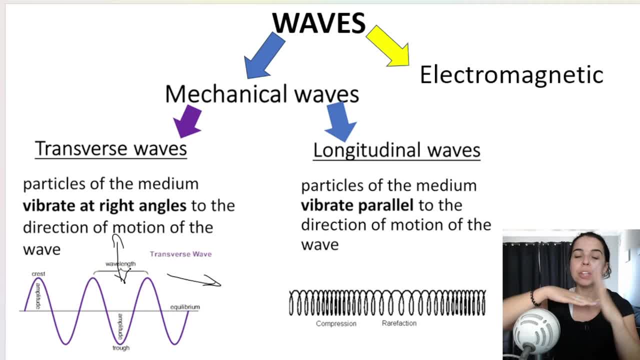 at right angles to the direction of motion of the wave. Longitudinal waves are different. The particles of the medium vibrate parallel to the direction of the motion of the wave. So each little particle is vibrating like this And the wave travels like this. So think of like.